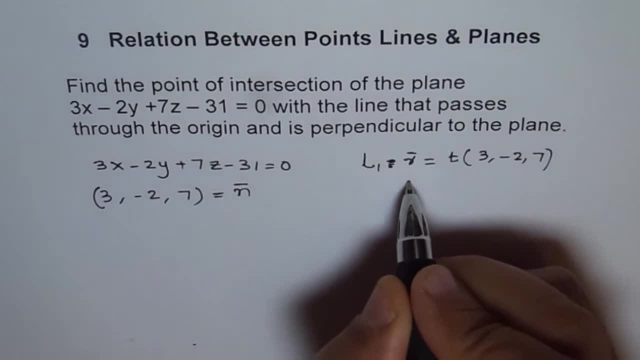 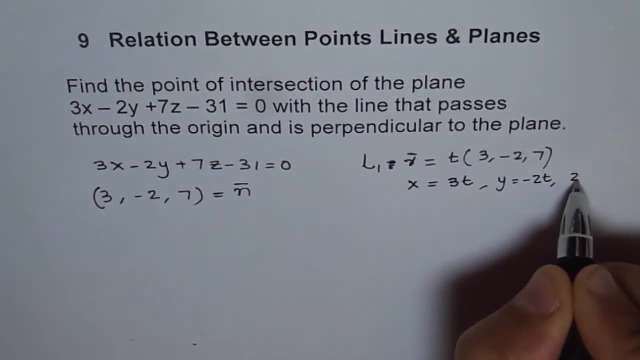 a general point on the line is what A general point on the line will be: x equals to 3t, y equals to minus 2t and z equals to 7t, right? So if this line has to intersect the plane? 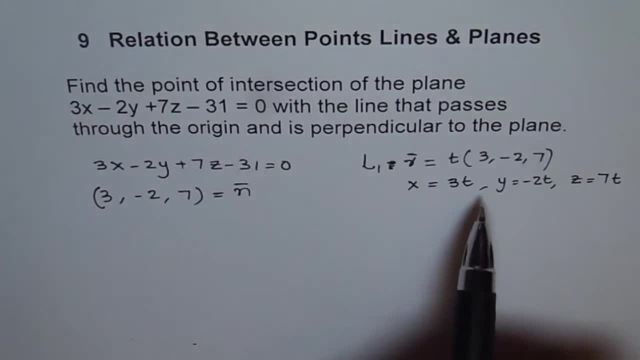 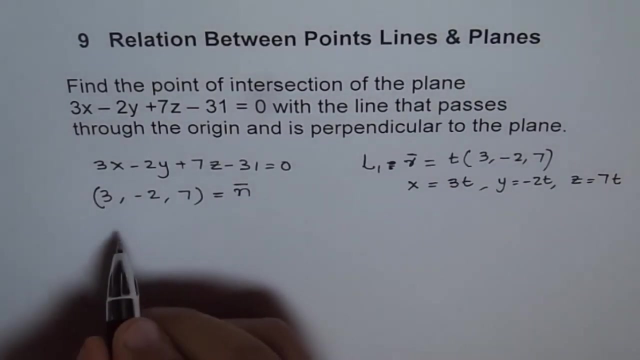 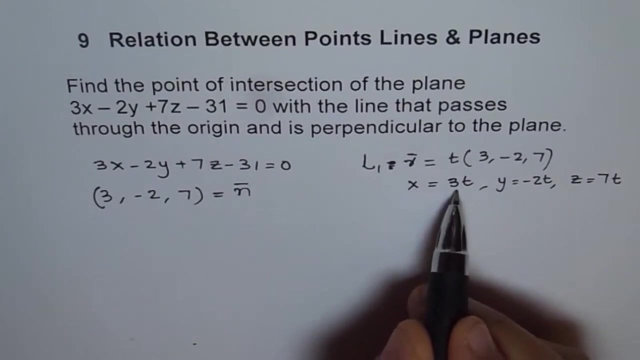 then they will have common points. That means these x values, when substituted into the equation of the plane, should give us some value of t, And then from there we'll find the point of intersection. So that's what we will do it now. So the equation is: 3x minus 2y plus 7z minus 31 equals to 0, less sub x is 3t, y is 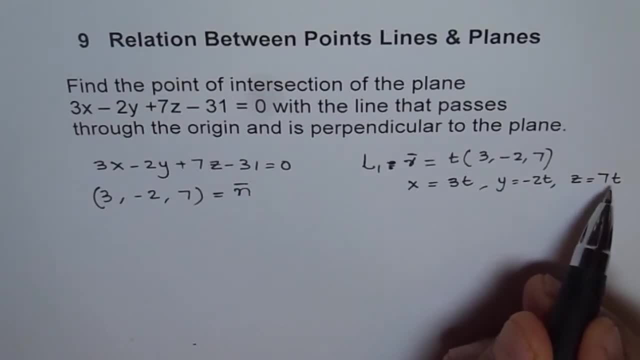 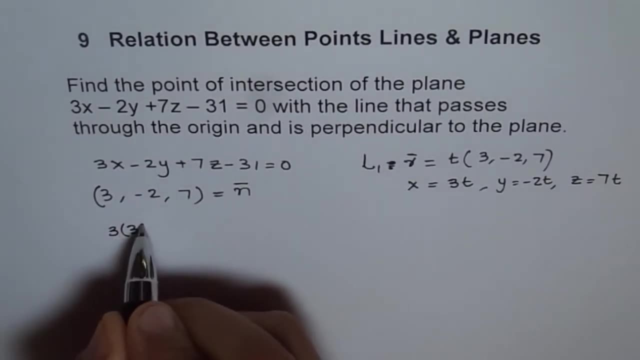 minus 2t and z is 7t. And then see what do we get? So we get 3 times 3t and this one is minus 2 times minus 2t, and then we have plus 7 times 70. 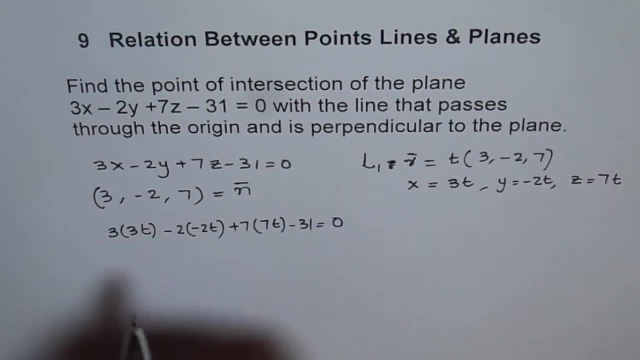 minus 31 equals to 0. This gives us 90 minus minus minus becomes plus 40 plus 49t. Let's take 31 to this side, so we get equals to 31.. So let's add them: 9 plus 4 is 13,, and 13 plus 49 gives us 62. So we get 62t equals to 31.. Or t is. 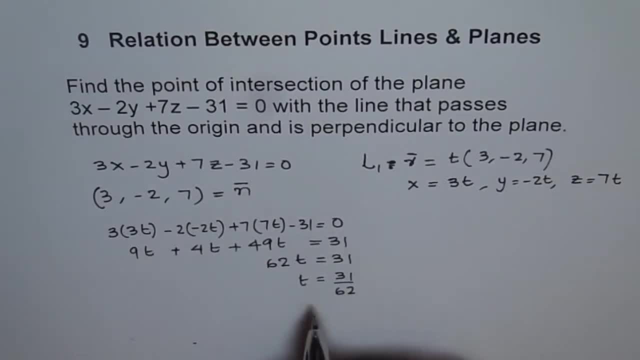 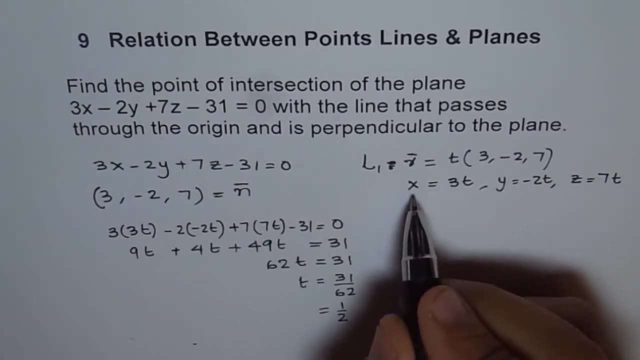 equals to 31 over 62, which is equal to half. So that's the value of t which we got. So our point should be: x is equals to half of this, right. y equals to half of this And z is half of 7, right. So our point P of intersection will be okay. so we can write like: 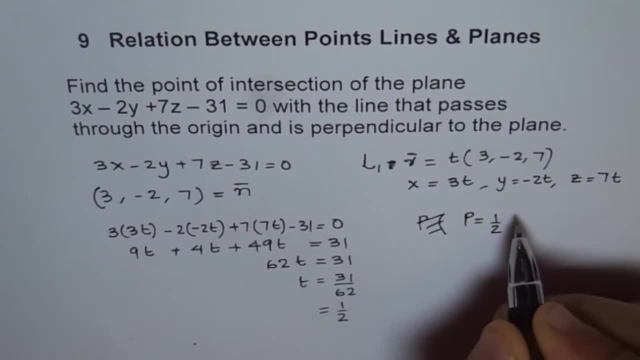 this first. Let's say point P is equals to half of. let me write it in two steps: t is half right, 3 minus 2 and 7.. So I can write this as: 3 over 2, minus 2. divided by 2 is minus 1, and 7 over 2,.